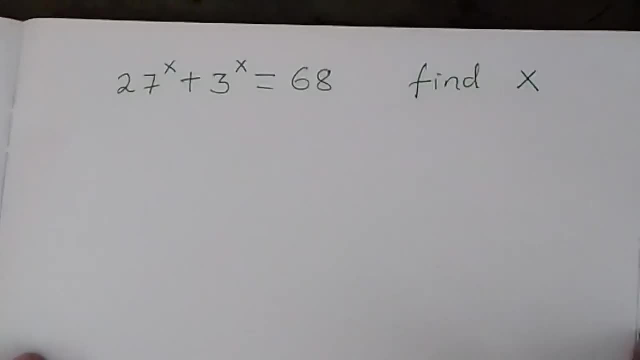 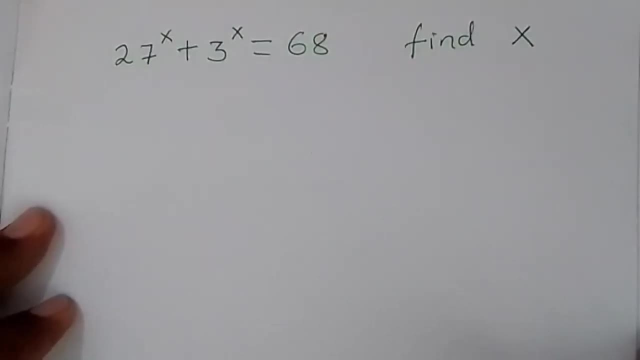 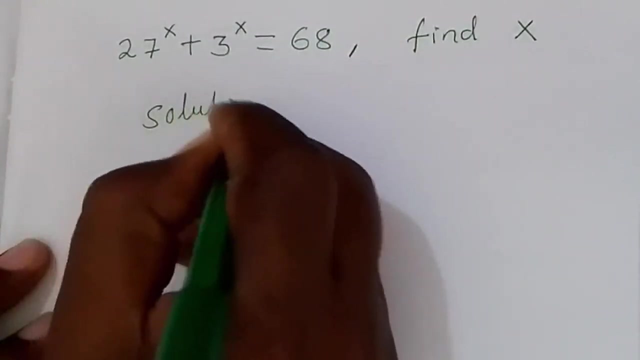 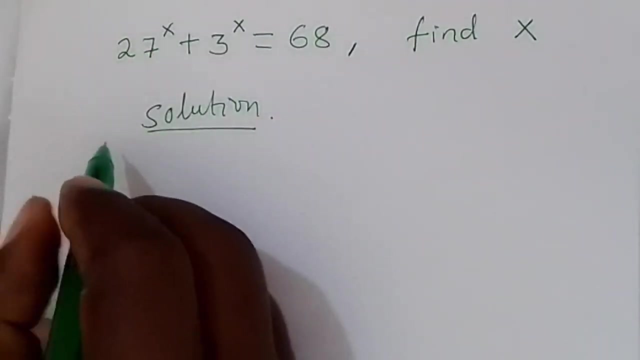 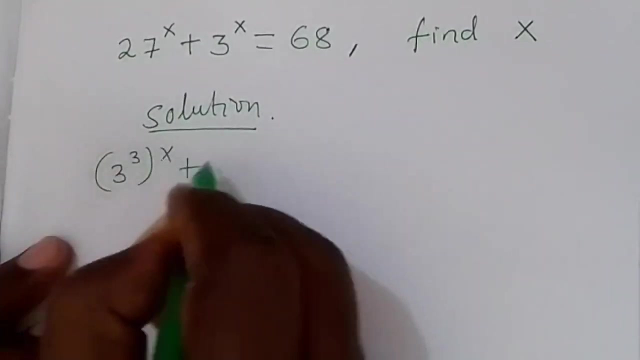 Aloha and welcome. How to solve this exponential equation: 27 to the power x plus 3 to the power x equals to 68.. Find x, Let us get started. Solution. Let us change the form of 27.. So we have 3 cubed to the power of 3 to the power x plus 3 to the power x equals to 68. 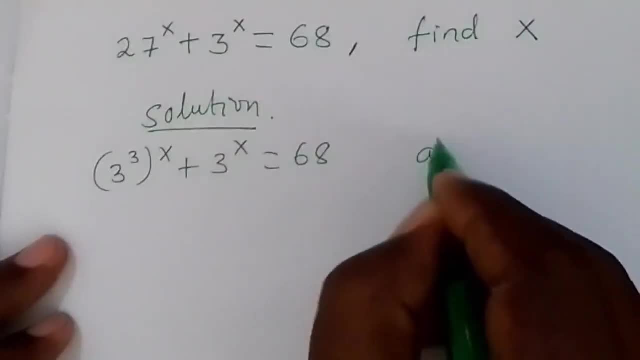 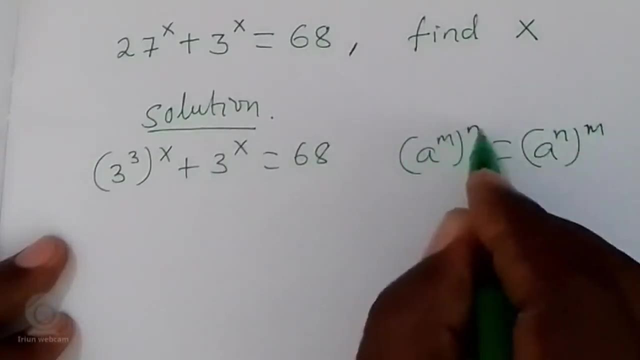 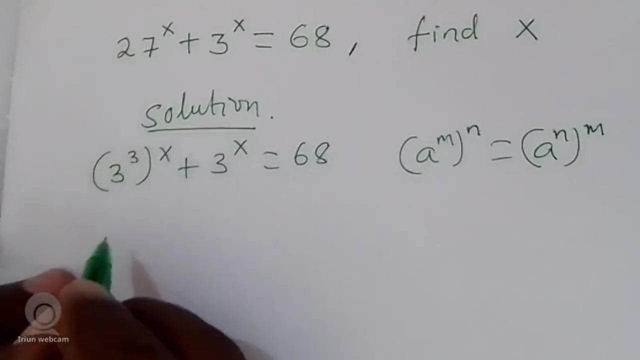 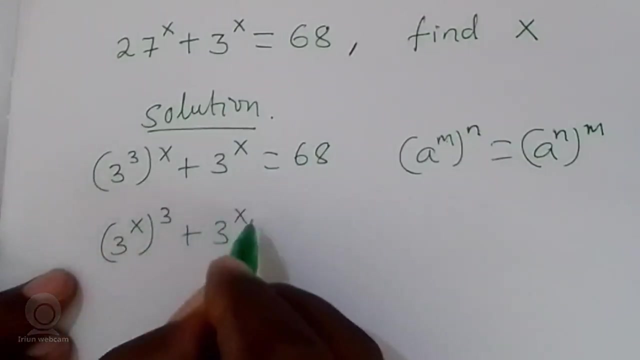 Apply this rule on the first term, that a raised to the power m to the power of 3 to the power x is the same as a raised to the power n to the power m. You swap these exponents Now by swapping 3 and x here. So we have 3 raised to the power x to the power of 3, cubed plus 3 raised to the power x equals to 68. 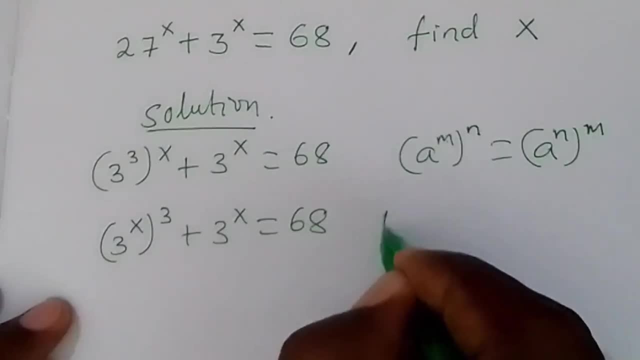 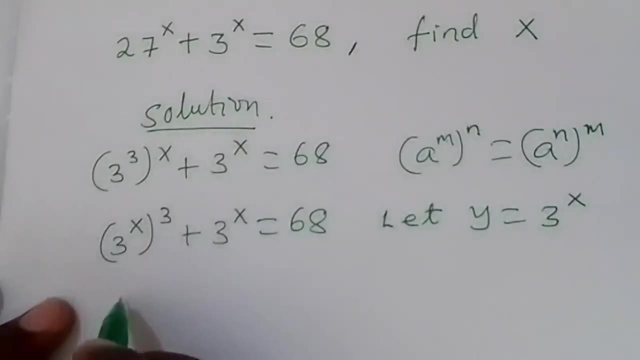 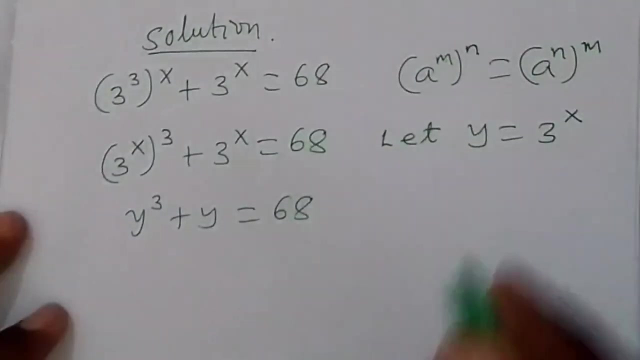 Now here let y be equal to 3.. Now y equals to 3. raised to the power x, By putting in y, we have y. cubed plus y equals to 68.. Now let us obtain: the factors of 68 are 17 times 4.. Now let us express this y here in terms of 17.. So y equals to 17y minus 16y. 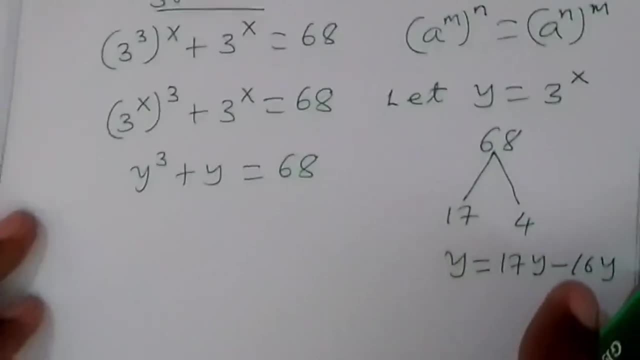 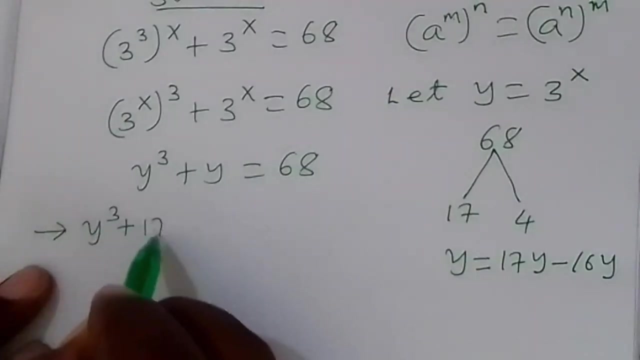 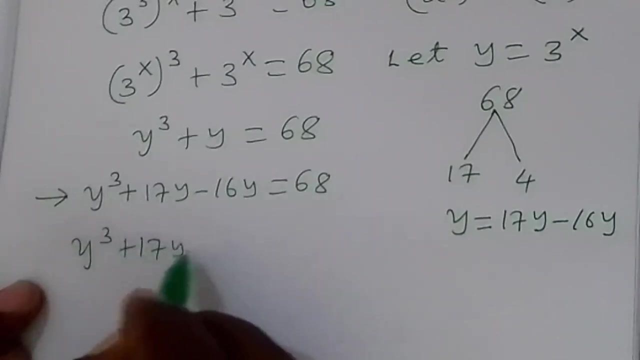 Now let us put in this new form of y Now. next, we have y cubed plus 17y minus 16y equals to 68.. Now let us bring all terms to one side of the equation. Now we have y cubed plus 17y minus 16y minus 68 equals to 0. 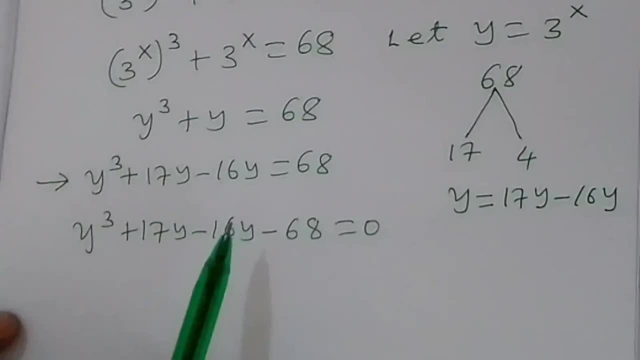 Now let us bring all terms to one side of the equation. Now let us bring all terms to one side of the equation. 17Y come back By rearranging, we have y cubed minus 16y plus 17y minus 68 equals to 0.. 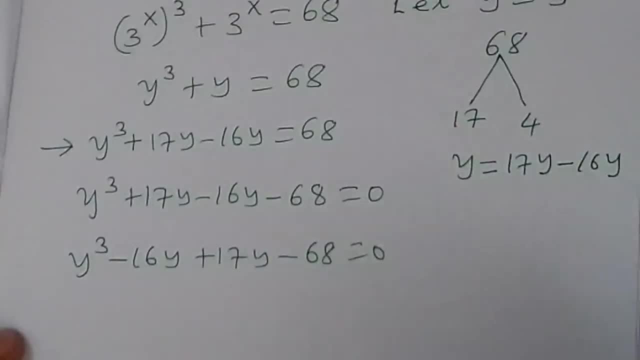 Now by same factorizing the first two terms And then the last two terms. In the first two terms, y is common, So we have y into y squared is equal to zero. So we have y and z equals to zero. Now let us do the same thing again. 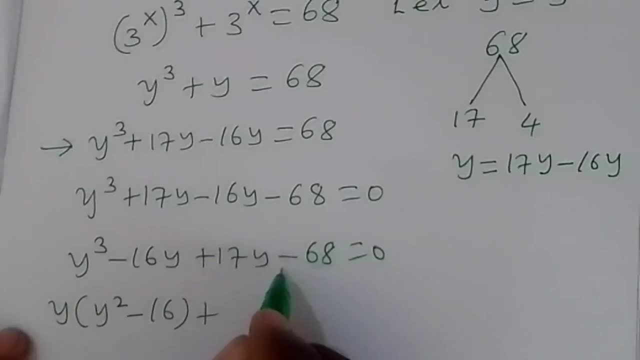 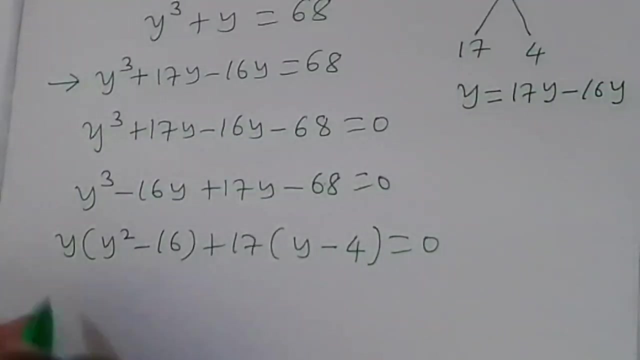 add minus 16 plus 17 is common between the last two terms, so we take it out. so 17 into y minus 4, because 17 times 4 you get 68 equals to 0.. now 16 can be written as 4 squared, so we have: 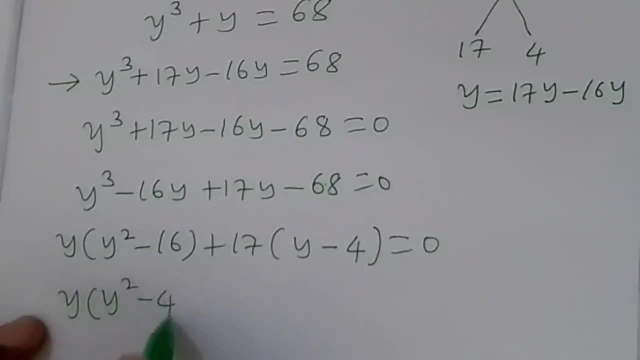 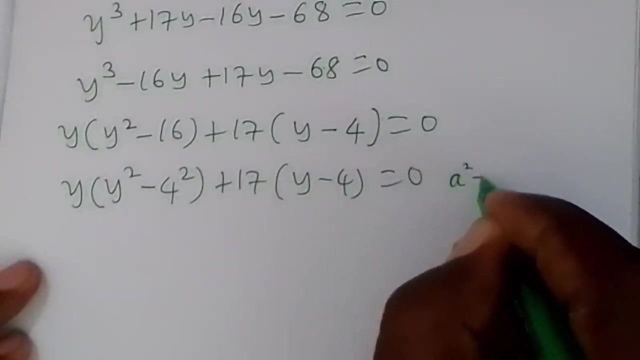 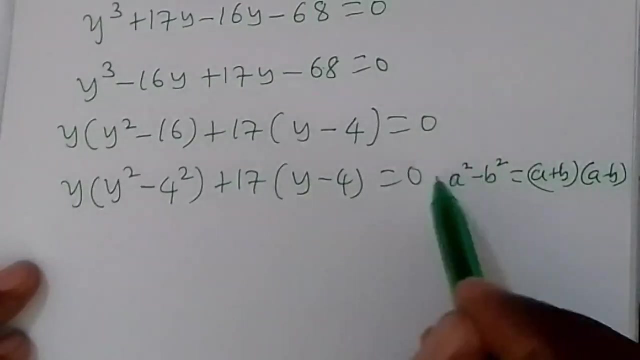 y into y, squared minus 4, squared plus 17 into y minus 4 equals to 0.. now, here apply this rule that apply this rule that a squared minus p squared is the same as a plus p into a minus p. so we are going to apply the difference of two squares on this factor here now. next, we have 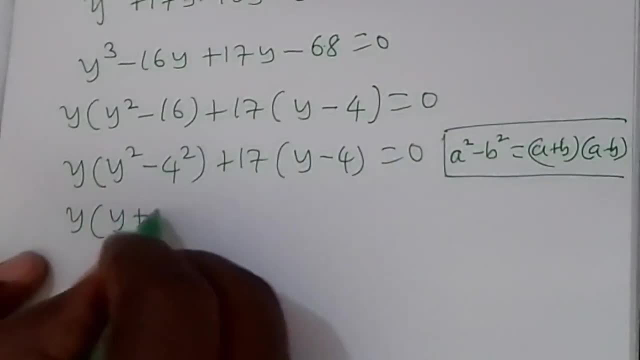 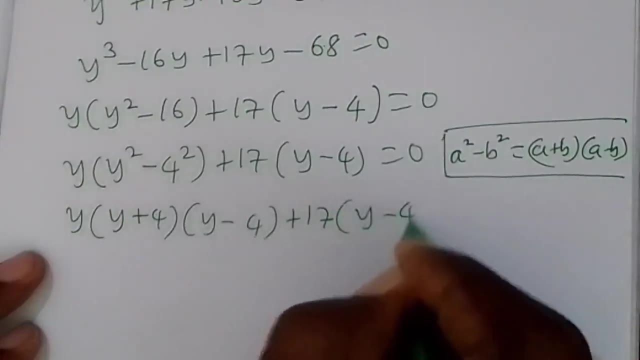 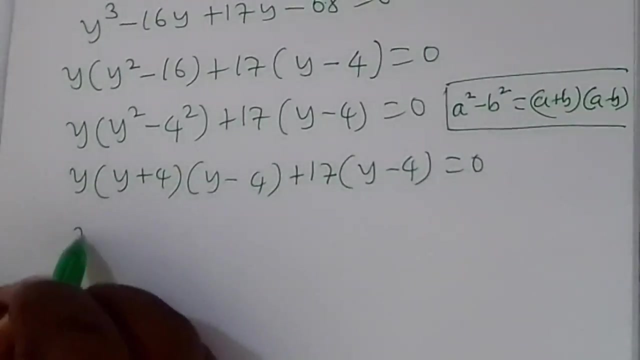 y into y plus 4 into y minus 4. plus 17 into y minus 4 equals to 0.. now y minus 4 is common. take it out between the two terms. so we have y minus 4 into y. now we remain with this y here. times y plus 4 into y plus 4. 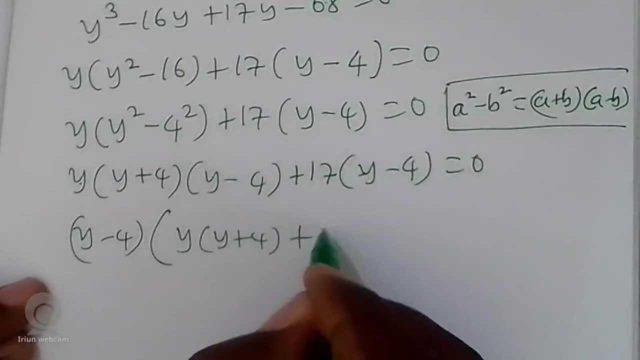 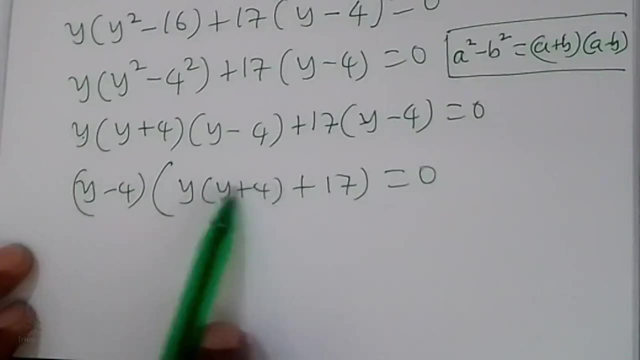 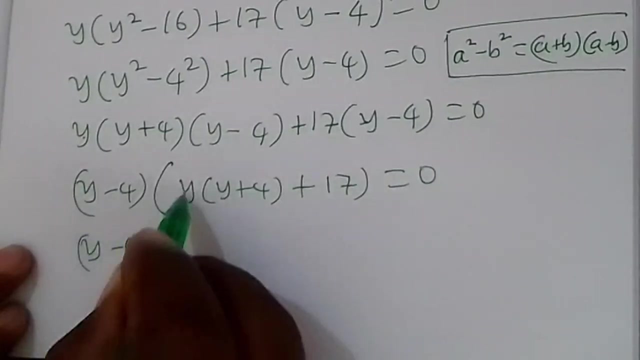 now, here we remain with 17 when we take out y minus 4. so plus 17 equals to 0.. now let us expand these two terms of the next factor, of the next major factor. so we have y minus 4 into y times y. you get y squared y times 4. you y times y. you get y squared y times 4 you. 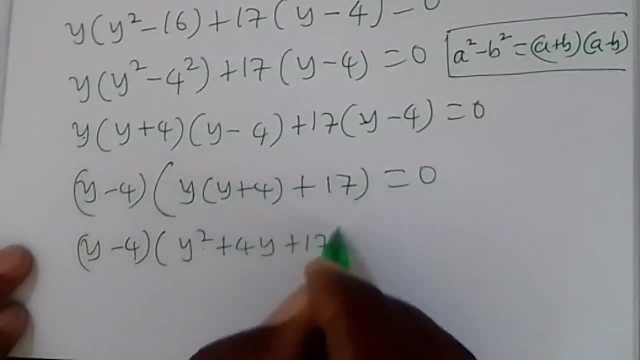 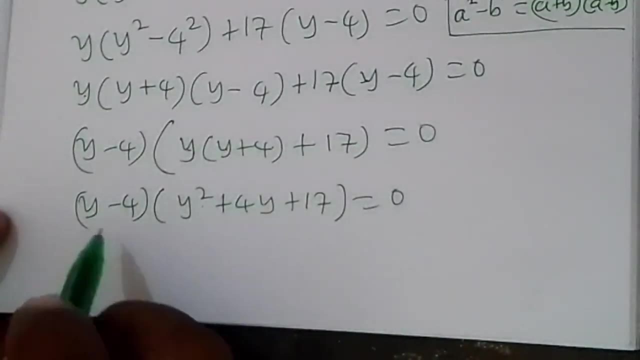 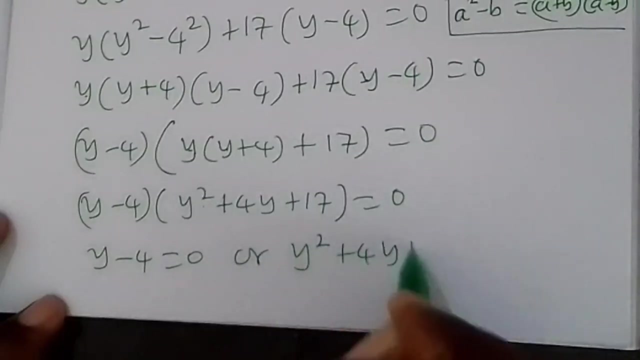 get plus 4, y plus 17, this one here equals to 0.. now we have two factors here, so it implies that y minus 4 equals to 0, or y squared plus 4, y plus 17 equals to 0.. now let us have this: 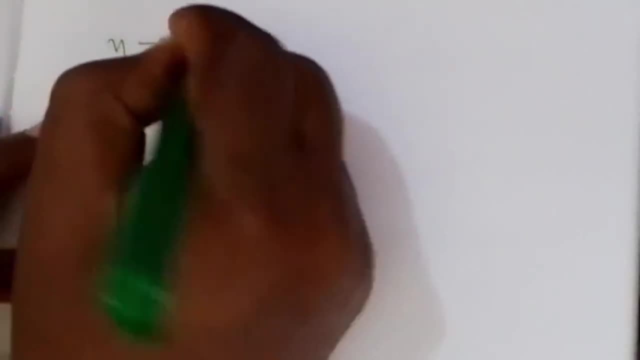 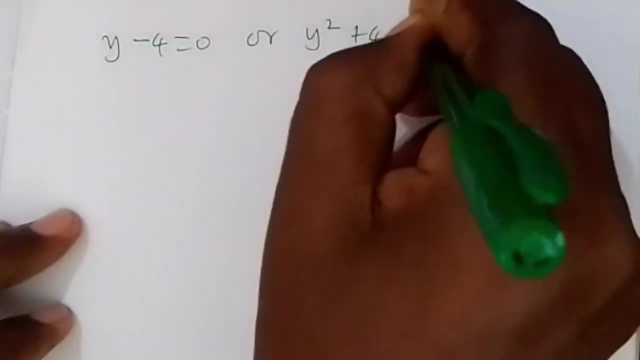 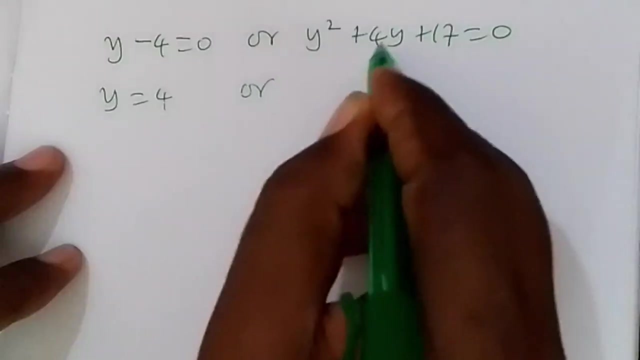 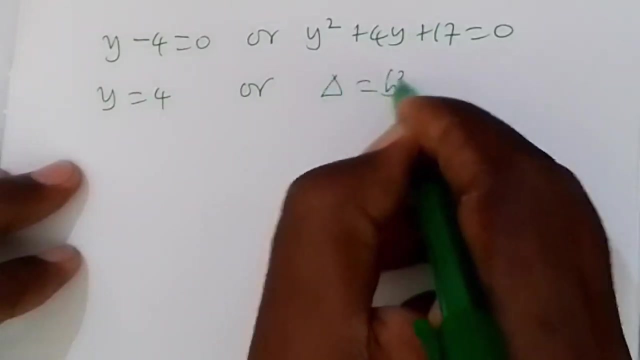 now we have y minus 4 equals to 0, y squared plus 4, y plus 17 equals to 0.. which means that to 4, or for this one, let us check for delta. to test the weather, you can get three solutions. now delta is given by p squared minus 4ac, in which a equals to 1. deleting coefficient. 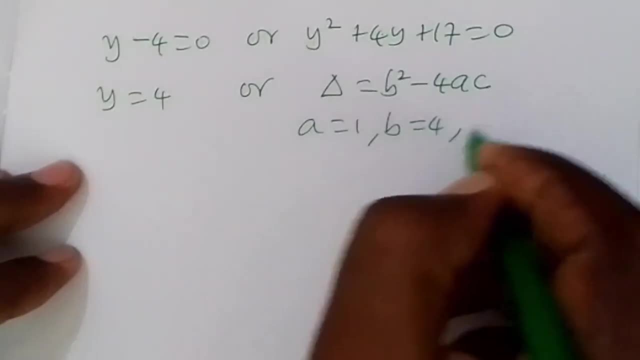 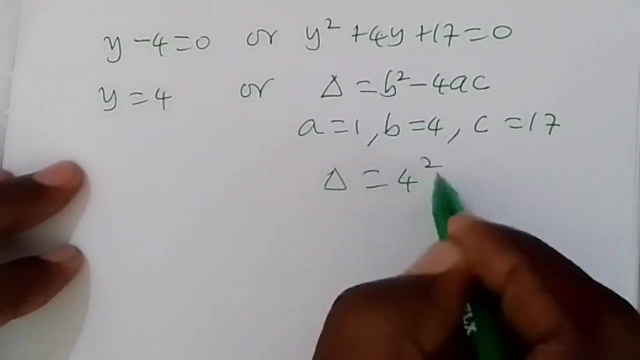 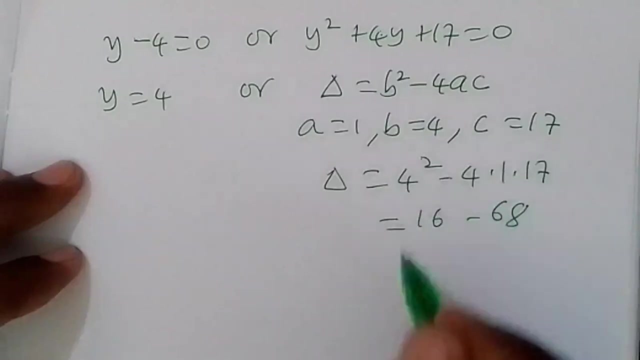 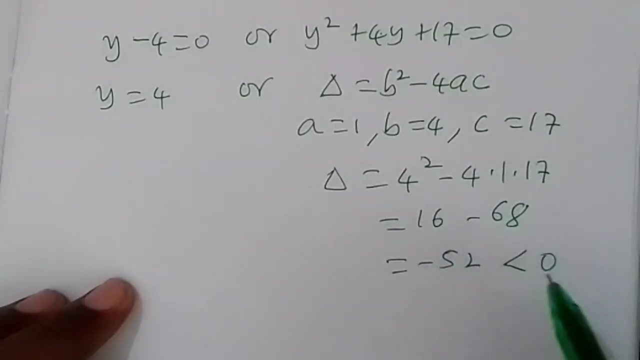 p equals to 4. the coefficient of y and c, which is the constant term, equals to 17. now, by plugging in the parameters, delta equals to 4 squared minus 4 times 1 times 17, which gives us 16 minus 68. now this one gives us minus 52, which is less than 0. the value of delta. 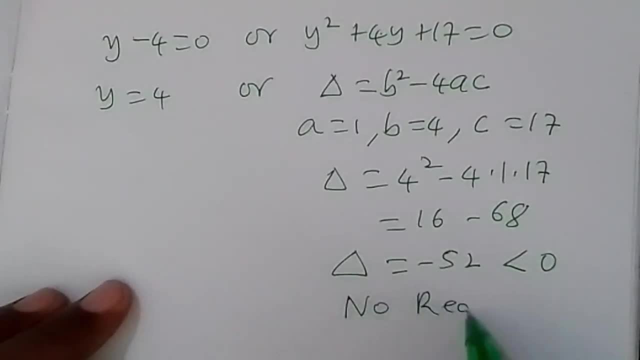 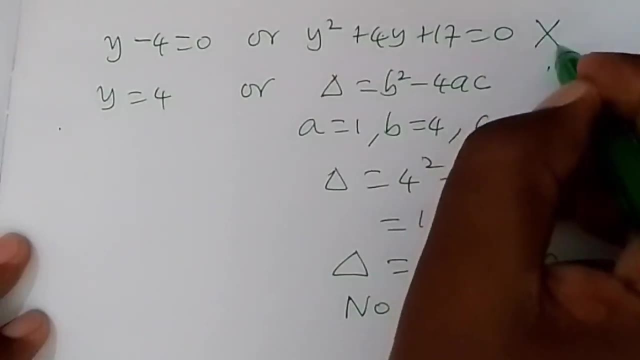 which means that no real roots because of this negative here. so this case should be less than zero because of this negative here. so this case should should be less than zero because of this negative here. so this case should be less than zero because of this negative here. so this case should be, it should be rejected. 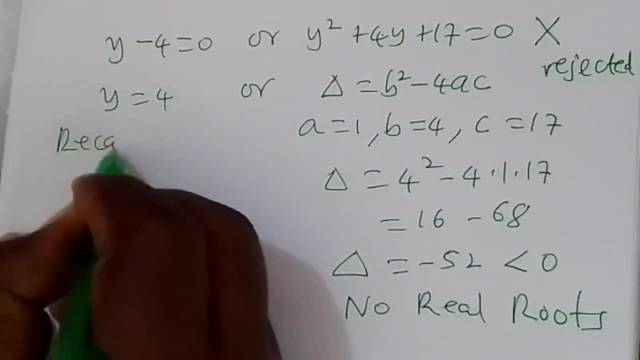 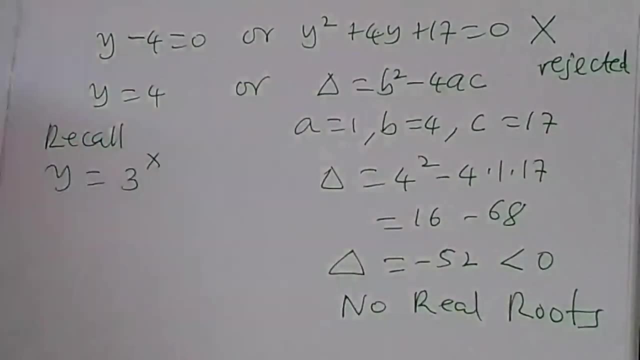 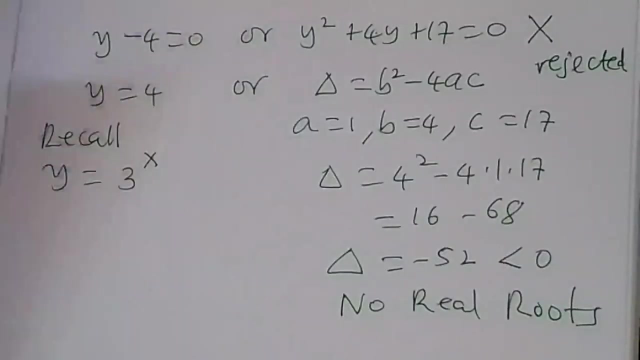 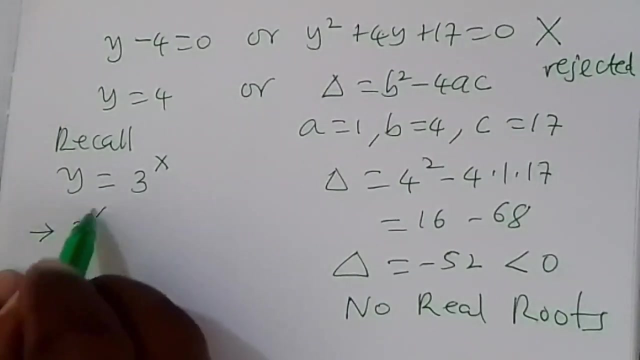 now for this one here. recall: y equals to 3 raised to power x. from here we say it: let y be equals to 3 raised to power x. and we know that y equals to 4. it implies that y equals to 3 raised to power, x equals to 4.. 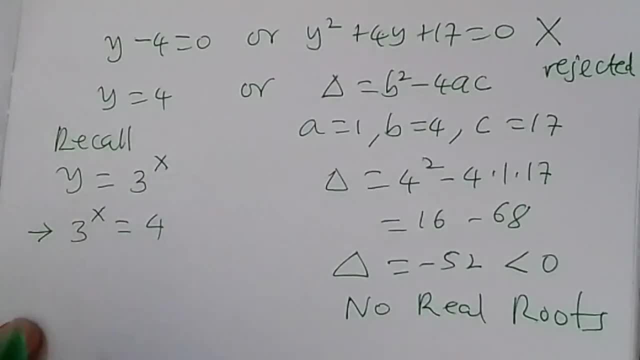 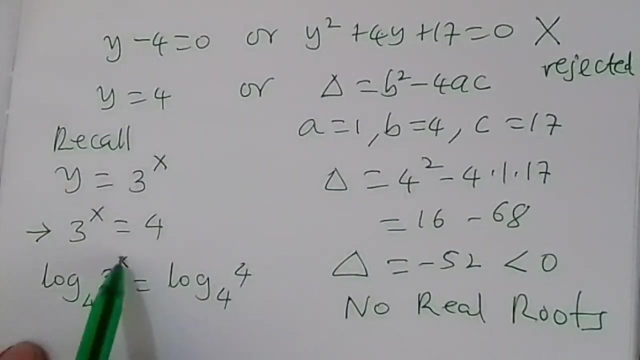 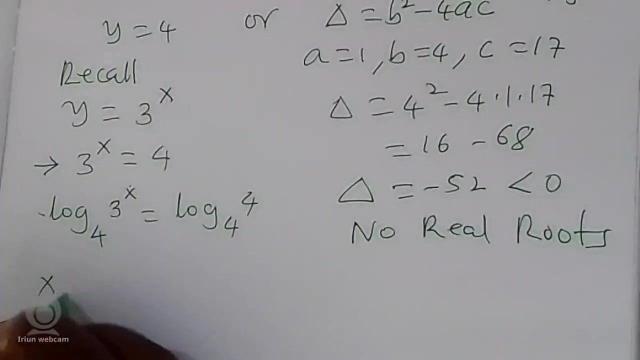 now let us take logarithms to base 4. so we have the logarithm of 3 to power. x to base 4 equals to the logarithm of 4 to base 4.. now this exponent comes here by the application of the power rule. now this one becomes x log. 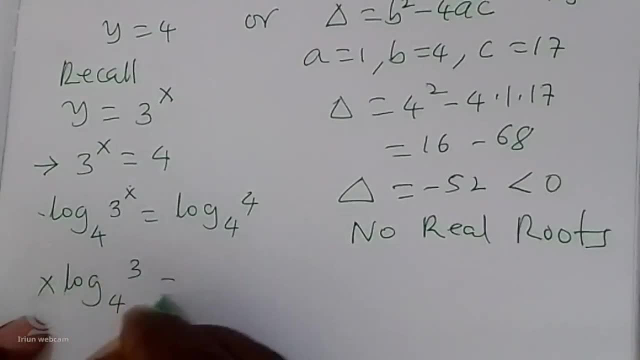 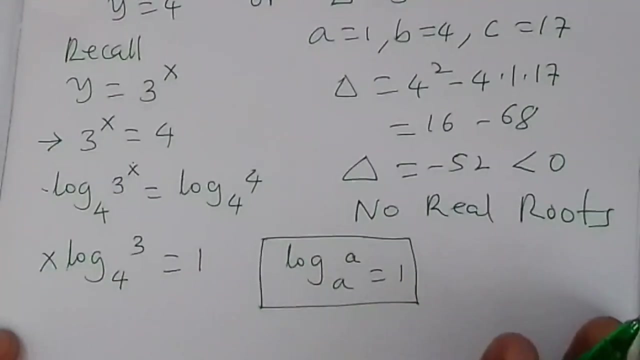 3 to base 4 equals to now this one becomes 1. by use of this relationship that the logarithm of a to base a equals to 1, free path rule. now here let us divide both sets of the equation by the logarithm of 3 to base 4.. 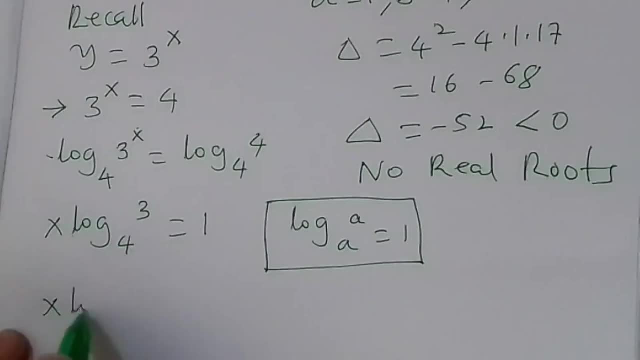 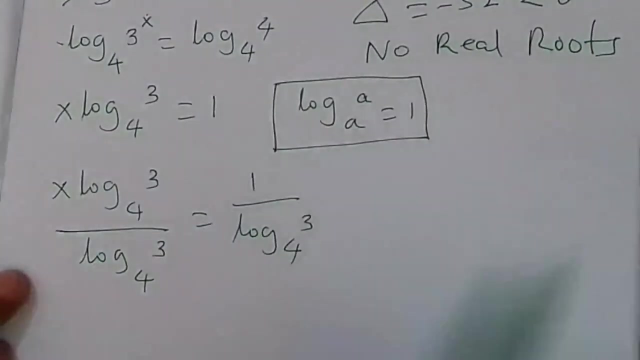 so we have x. log 3 to base 4 divided by log 3 to base 4 equals to 1 over log 3 to base 4.. So we've redoth both sets by log 3 to base 4, so this one and this one cancels. so we have x equals. 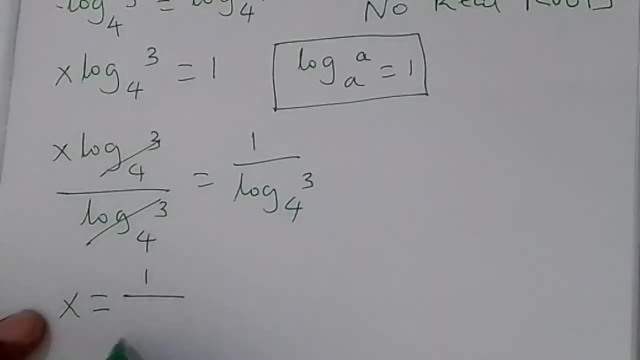 to 1 over log 3 to base 4.. Now Let us apply this rule that x is missing, percent of these valuesけど there's not just one thing missing in the equation, it const performing this equation. interesting, If i sum this. So we have x. 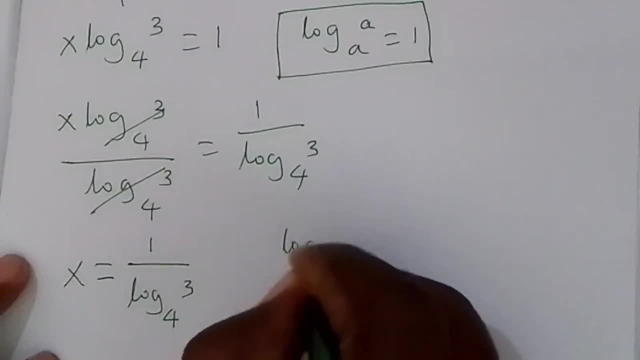 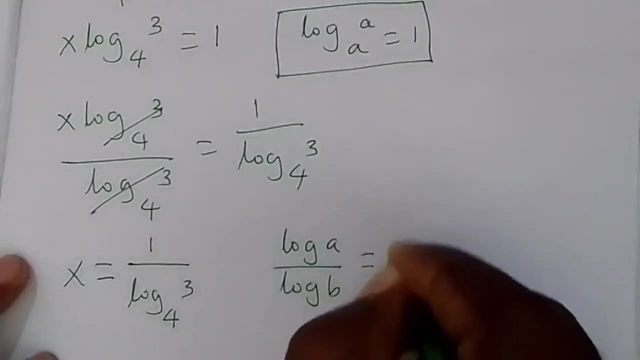 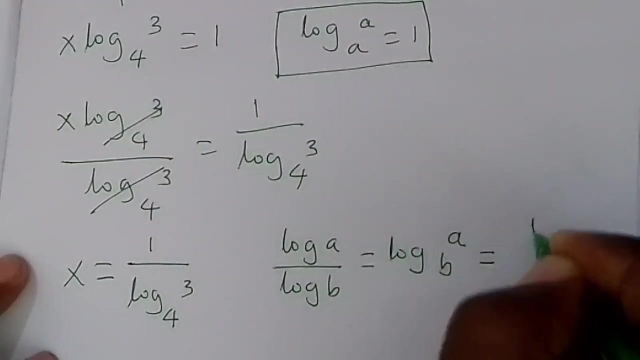 Now let us apply this rule, that that the logarithm of a over the logarithm of p is the same as the logarithm of a to base p, which is the same as 1 over the logarithm of p to base a, the so-called change of base. you can see. 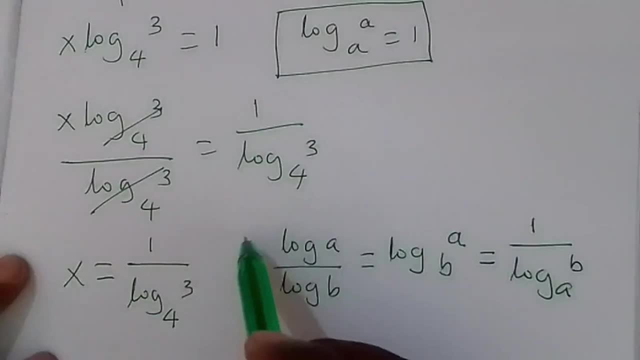 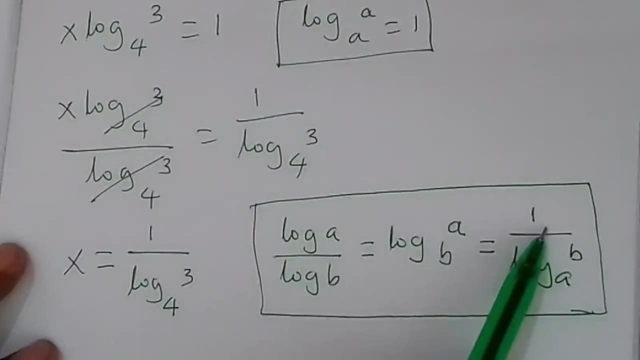 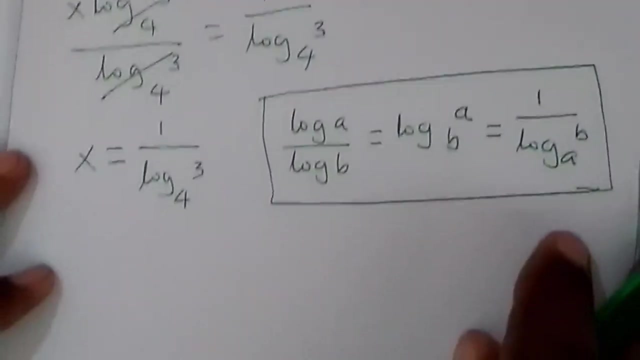 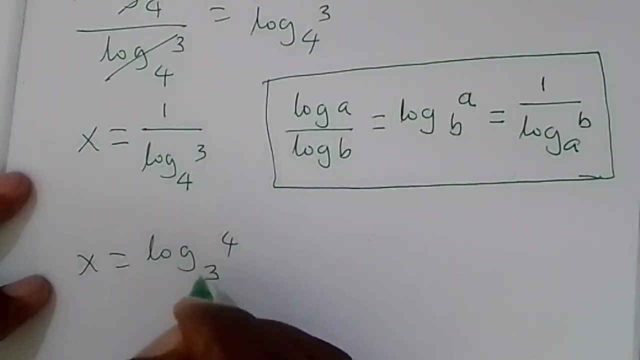 how the best anti-argument swaps. so this one is called change of base rule. now, by the progression of this rule, then we are going to move from here to this form. therefore this one becomes, by moving from this form to this one, so we have x equals to the logarithm of 4 to base 3. 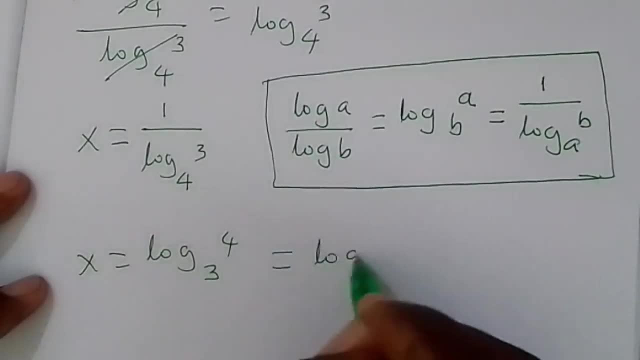 which can be written as logarithm of 2 squared, because 4 is the same as 2 squared to base 3, by use of the power rule in which this exponent comes here. so this one is the same as 2. log 2 to base 3, which means that x. 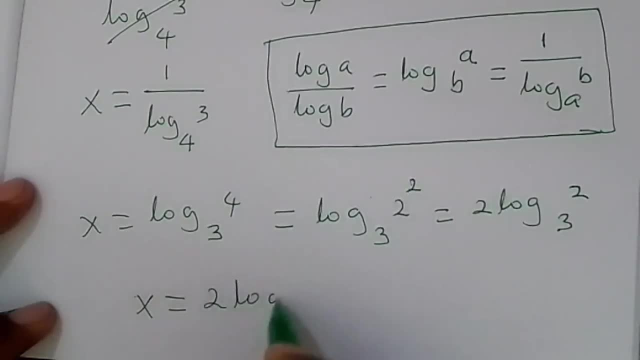 equals to 2. log 2 to base 3 and that is it. thank you for watching. subscribe to my channel and turn on the notification bell to get new updates. when i upload new videos, don't forget to smash the like button, share and comment below to make this video with many people.